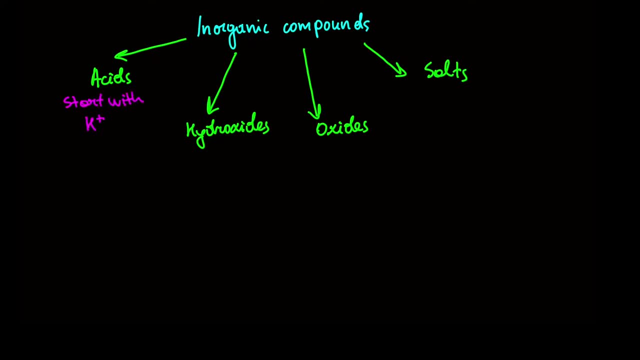 with H plus ion in their formulas, For example HCl, H2S, H2SO4, and so on. Next are hydroxides. All hydroxides, All hydroxides end with OH minus ion, For example NaOH, CaOH times 2, and AlOH times. 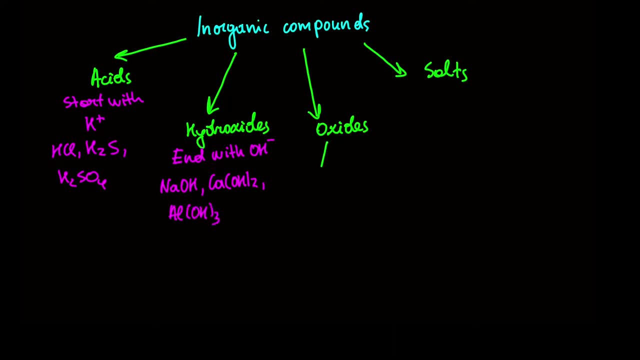 3. Let's talk about oxides. Oxides can be divided into two major groups: Basic oxides and acidic oxides. We can identify oxides very easily because they are always composed of only two elements. Now they are also called metal oxides because they have metal in their composition. The 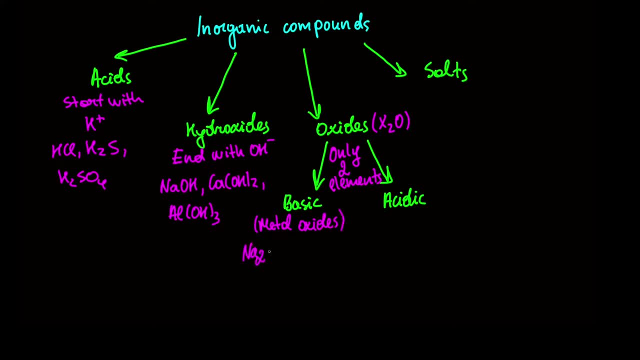 basic. accordingly, The basic oily Pam platanate makes comes as Na2O-CaO-Ni2O3.. As you see, all basic oxides are made from two elements. What is made of each one is metal, and Oxford is made of講 CG. 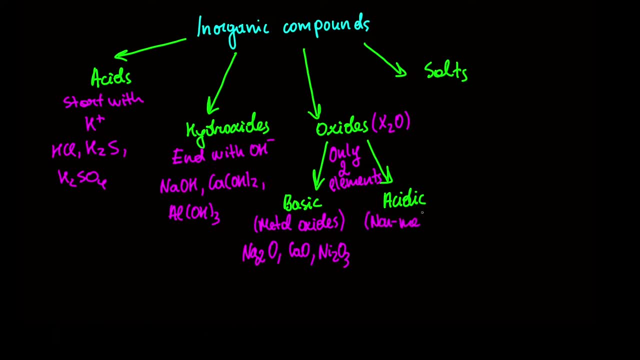 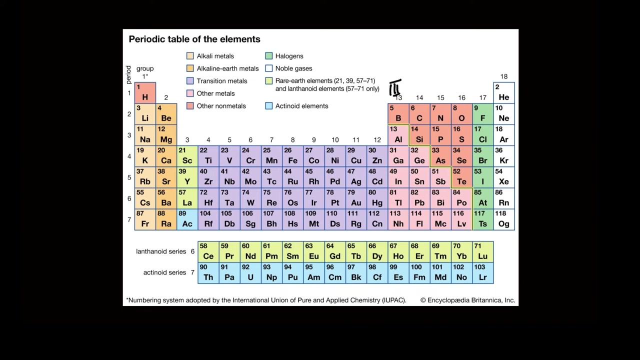 oxygen For acidic oxides. we have non-metal and oxygen in their composition, For example CO2, SO2 and B2O5.. Now which elements are metals and which are non-metals? I have a periodic table here, and in the third A group under boron, you should see a black. 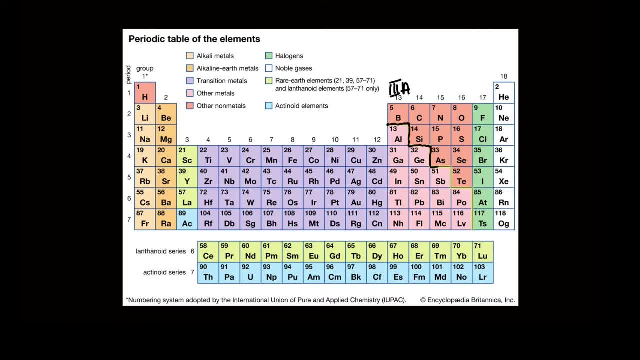 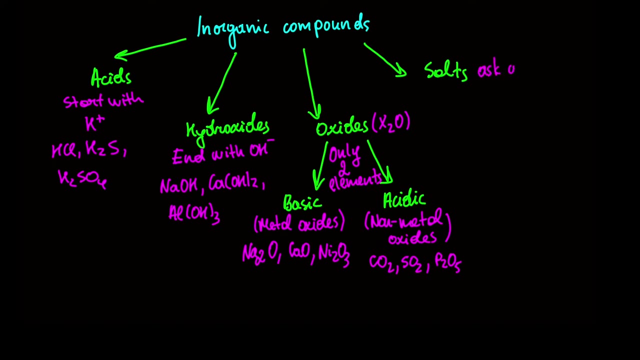 line that goes throughout A groups in the periodic table and looks like a staircase. On the left side of that line resides all metals, and on the right side you have all non-metals. Lastly, there are salts. The easiest way to discern which compound is salt and which is not is to ask yourself: 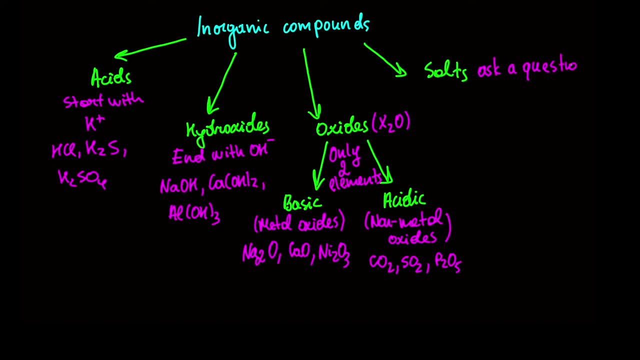 a question: Is this compound an acid, a hydroxide or an oxide? If the answer is no, then we are dealing with a salt, For example KCl. It's not an acid because it doesn't start with H, and not a hydroxide because it doesn't.